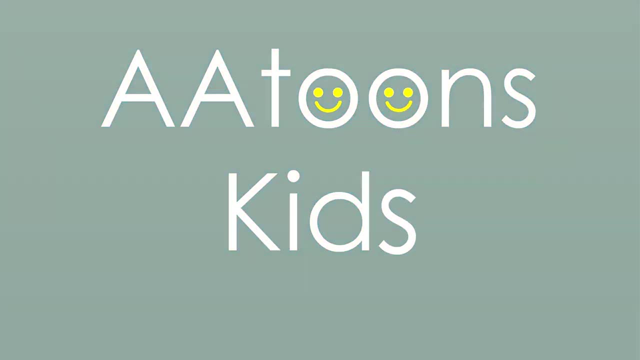 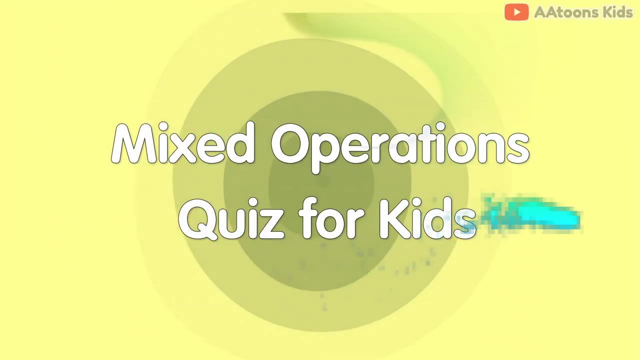 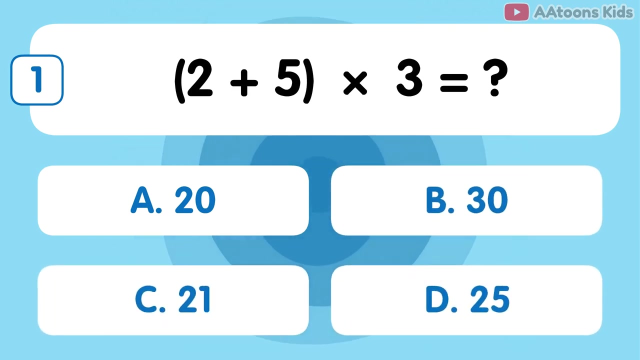 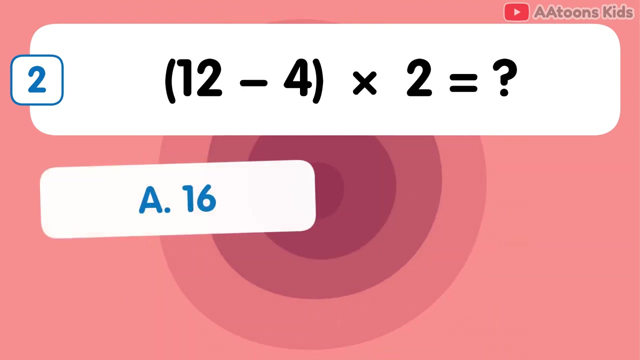 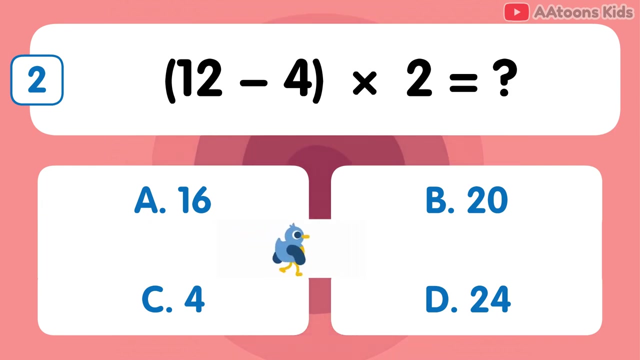 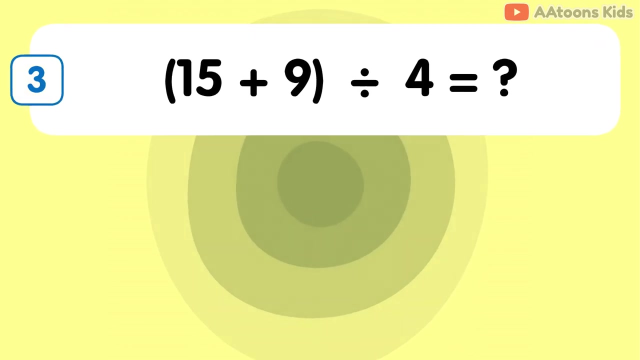 Mixed operations quiz for kids. 2 plus 5 multiplied by 3 is 21,. 12 minus 4 multiplied by 2 is 16,. 15 plus 9 divided by 3 is 21,. 20 minus 10 multiplied by 4 is 6,. 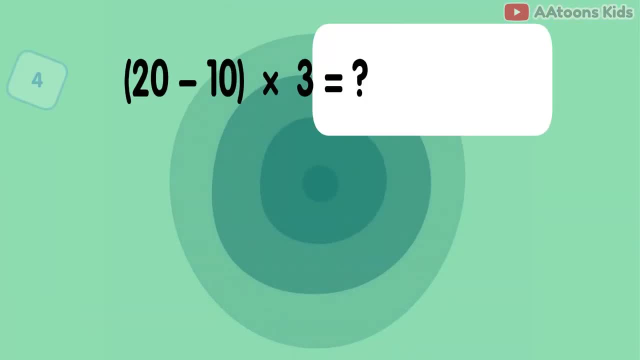 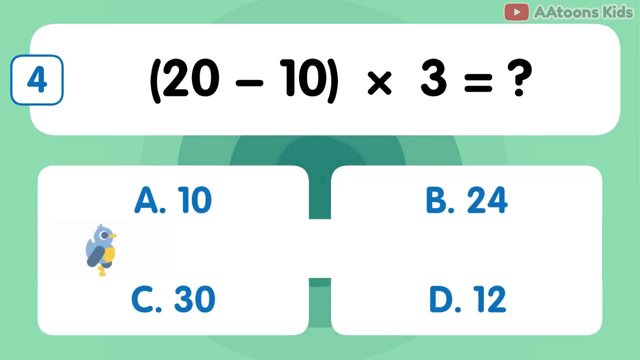 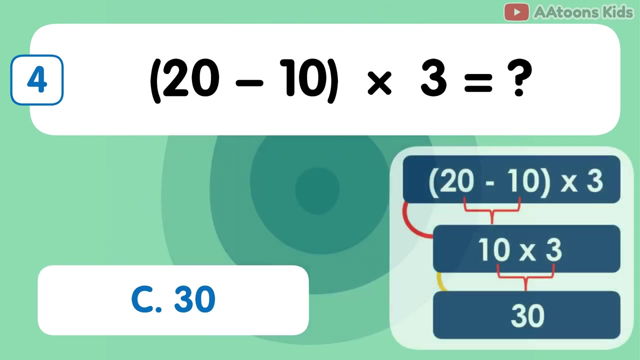 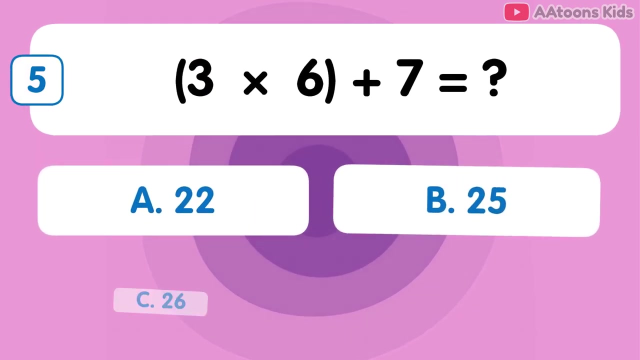 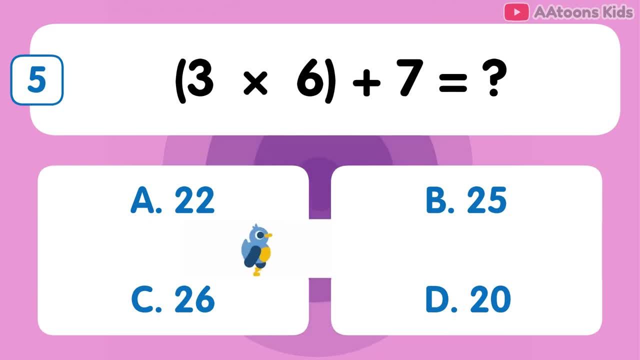 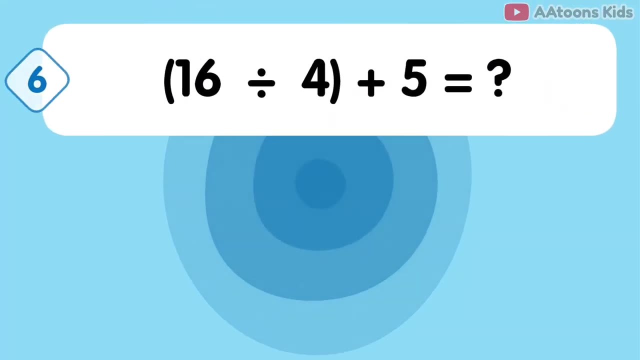 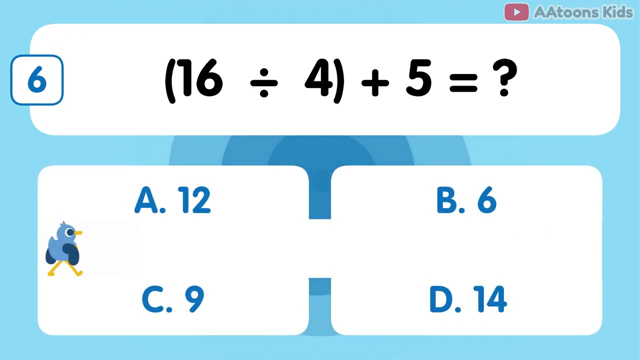 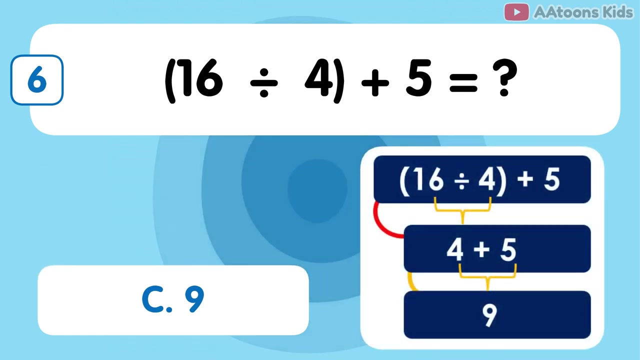 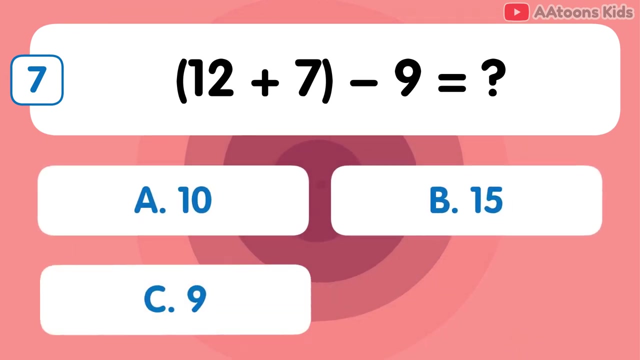 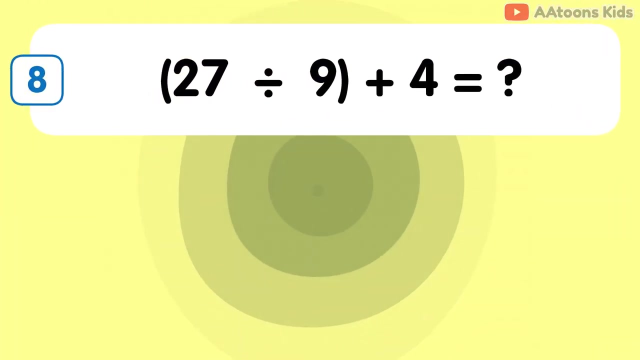 30.. 30.. 30, 30,, 50.. 30, 30, 30.. 25- 16 divided by 4 plus 5 is 9. 12 plus 7 minus 9 is 10. 27 divided by 9 plus 4 is. 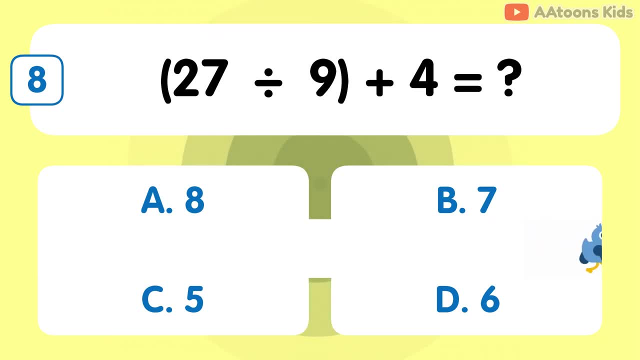 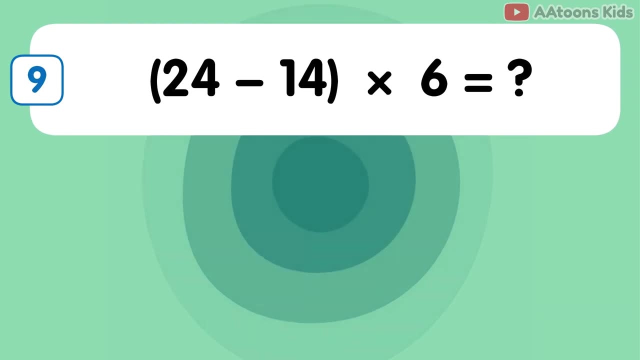 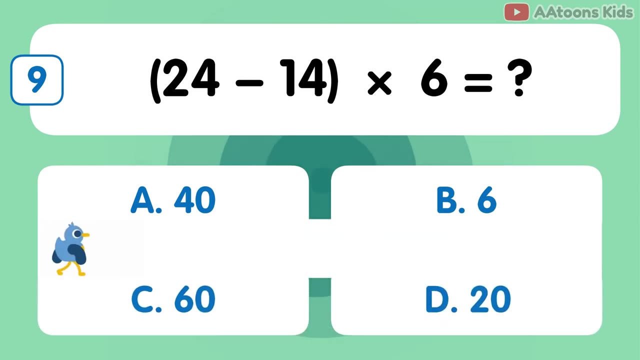 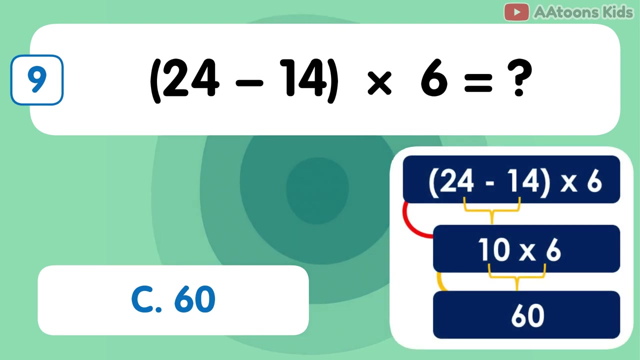 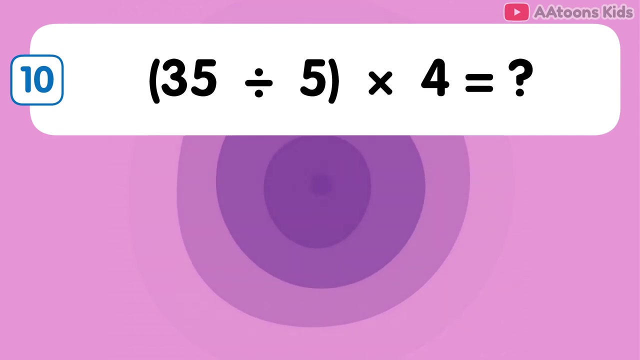 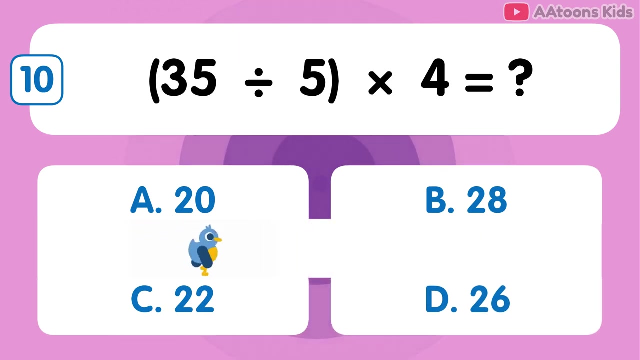 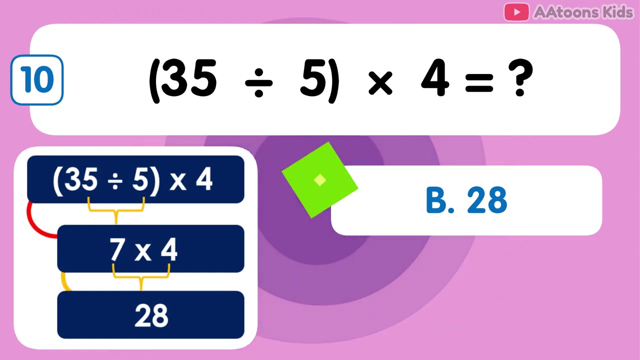 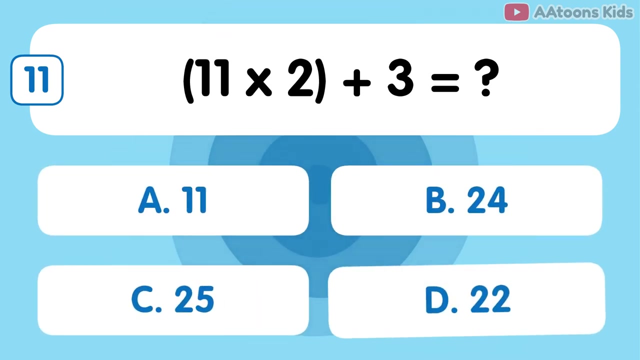 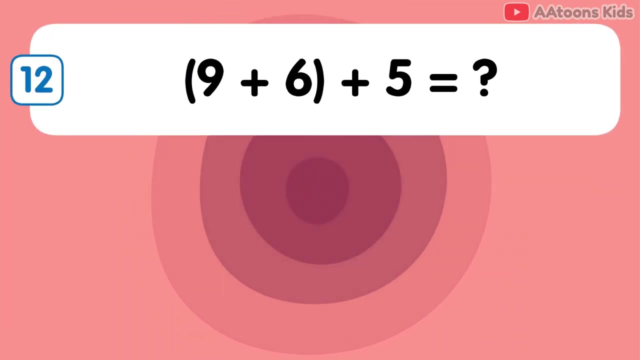 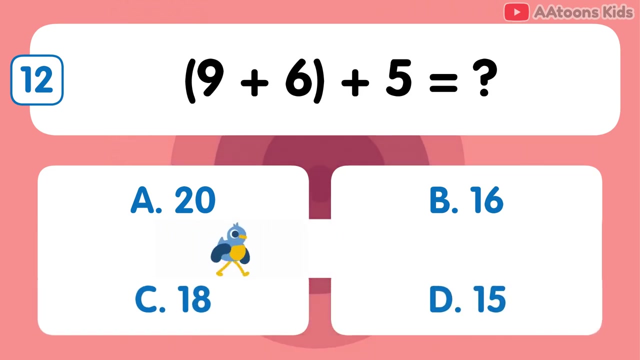 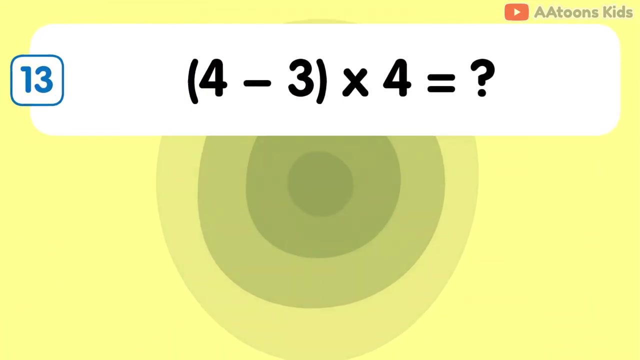 7, 24 minus 14 multiplied by 6 is 16. 35 divided by 5 multiplied by 4 is 28. 11 multiplied by 2 plus 3 is 25. 9 plus 6 plus 5 is 20, 4 minus 3 multiplied by 4 is. 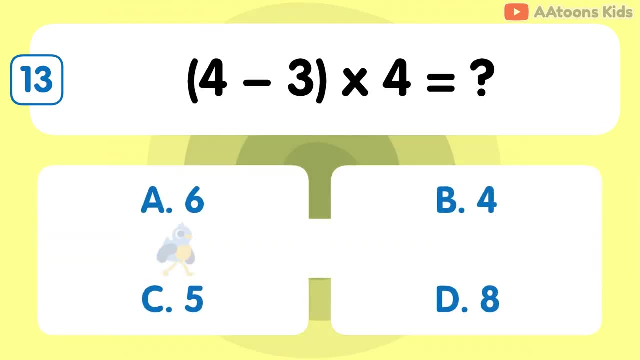 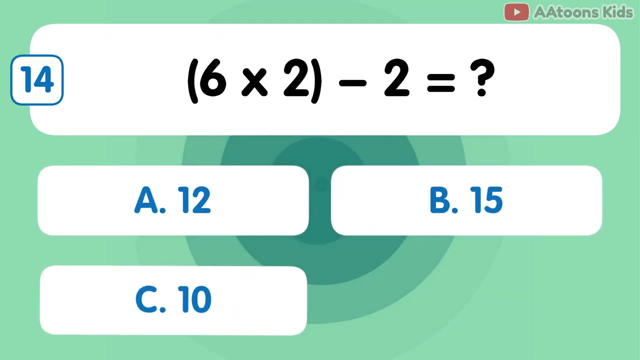 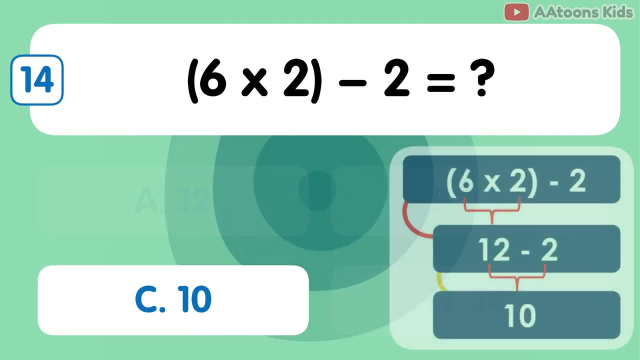 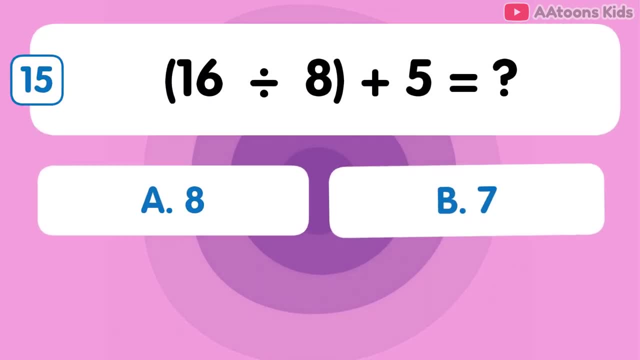 20, 20, 20, 20, 21, 21, 22, 23, 24, 25, 26, 27, 28, 29, 31, 32, 33, 32, 33, 34, 35, 36, 37, 38, 39, 40.